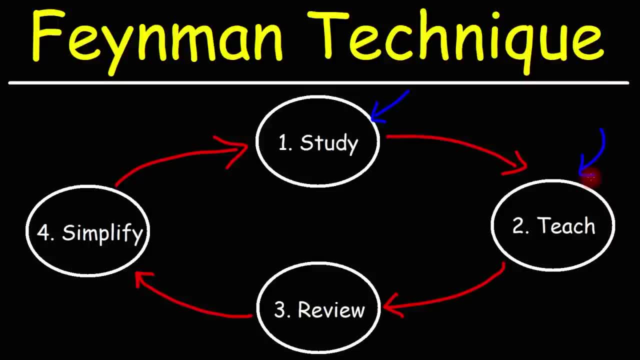 to yourself what you've learned. You could do this verbally or by writing down notes on a sheet of paper, But you can also even better try explaining it to someone else, Because if they don't get it, they'll ask you questions to see you know if you can help them understand it And if you can. 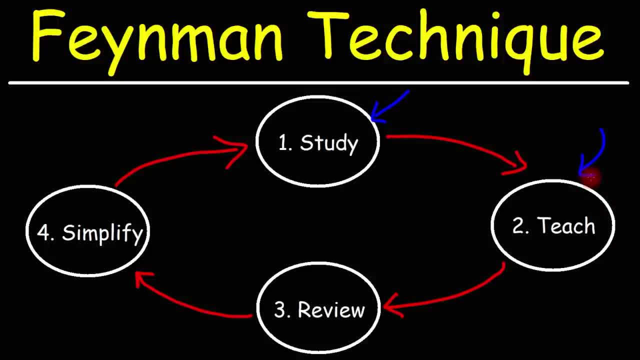 explain it in a way that they understand it, then that shows that you have a decent grasp of the topic. Now, I know this to be especially true in my case, Even though I've learned subjects such as chemistry and physics in high school. my understanding of these topics- they were greatly 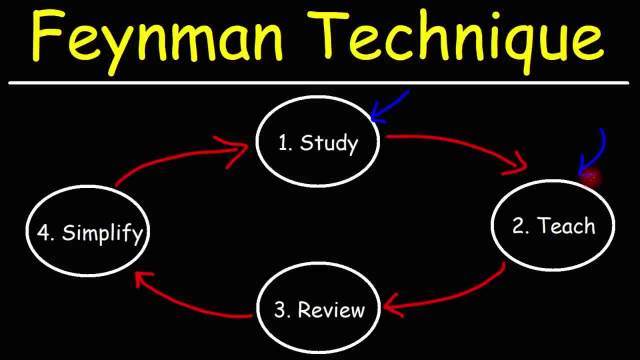 improved after I began working as a tutor, teaching it to other people. It's been said that as you teach others, you teach yourself. In fact, the process of explaining what you learn to yourself or someone else is very useful. It can help you to determine whether or not you understand your material to a reasonable degree, For instance. 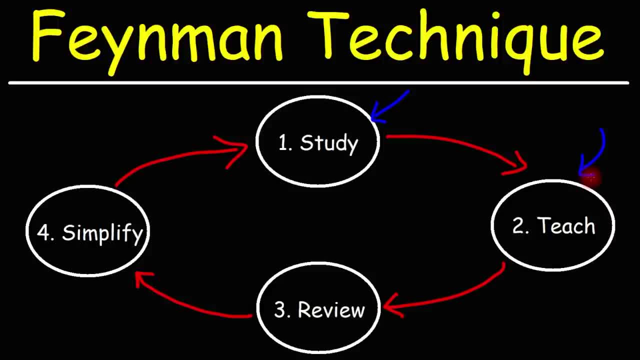 I've heard it been said that if you can't explain it well to someone else, you don't understand it yourself. Now the third step of the Feynman technique is to identify gaps in your understanding. After you try explaining the subject to yourself or someone else in step two, chances are you're. 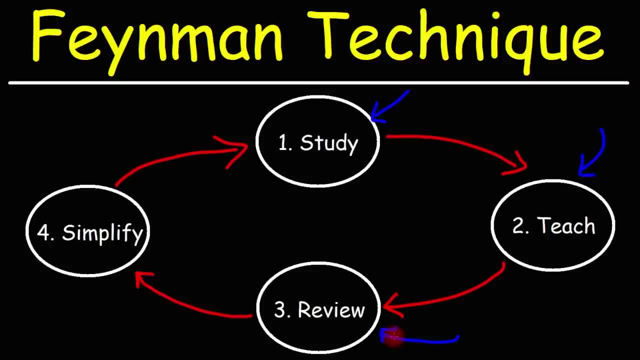 going to pick up on some gaps in your understanding that you didn't know were there the first time you learned the material. Once that happens, you want to go back and review the subject a second time to fill those gaps that you've identified. So whenever you're reading a book, or, let's say, if 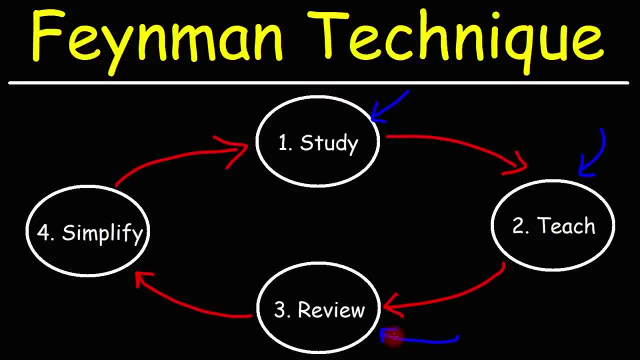 you watch a movie. whenever you do it a second time, you're going to be able to identify gaps in your understanding. Don't you notice additional details that you missed the first time you read the book or watched that movie? I know this is true for me. Therefore, whenever you learn anything new, it's 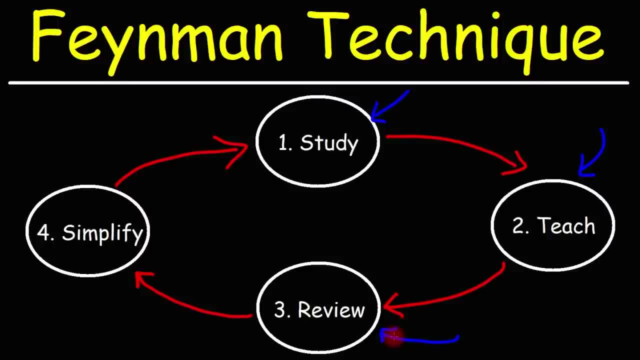 always good to review the material a second or third time to gain a better understanding of the subject, Because once you understand it, it's going to be difficult for you to forget it. I know in school what I like to do is I like to learn the material ahead of time, before the teacher teaches. 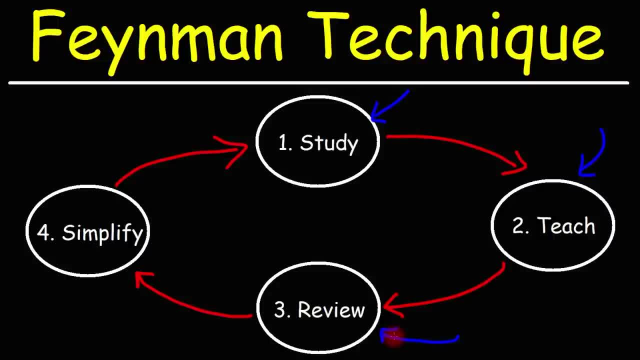 it in class, Because once I'm exposed to the material the second time, it deepens my understanding of the material. So anytime you review a topic, you look at it a second, a third or fourth time, you're going to gain additional details that you probably didn't notice were there before. So that third step: 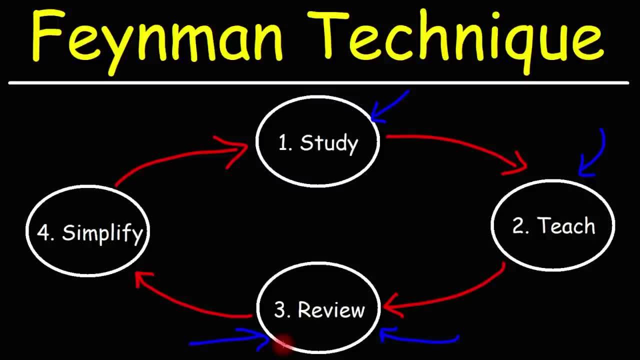 reviewing to like fill in the gaps of what you don't understand. that's part of the Feynman technique. Now, as you try to explain what you've learned to someone else in step two, when they ask you questions and if you feel like you can't answer it, that's how you can identify gaps in your 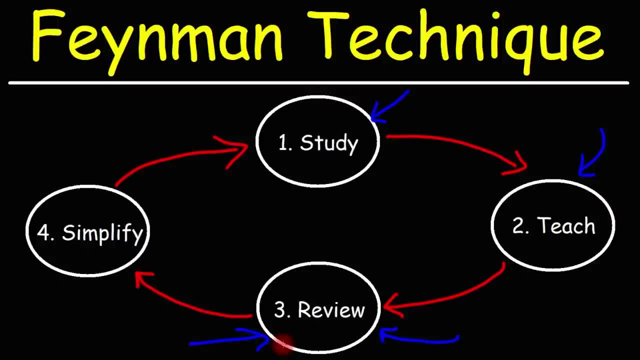 understanding. And that's when you go to step three to review the material again, to fill in those gaps that you've missed. Now the fourth step is to simplify your explanation. You want to understand the material so well that you can not only break it apart, down into its fundamental elements, but also make connections. 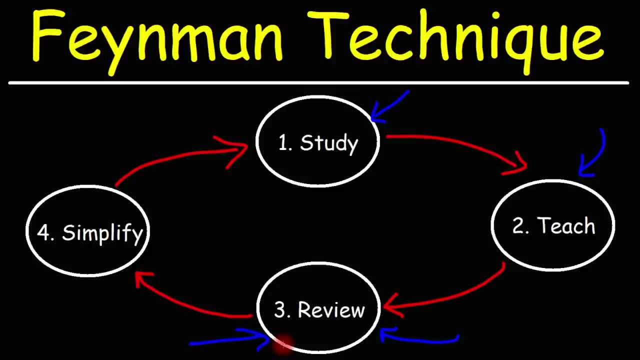 with other similar topics. Once you get to a point where you can explain it simply to a kid, that's when you reach a point where you've acquired a reasonable understanding of the subject. So whenever you wish to learn something new, or even understand something, try explaining it to. 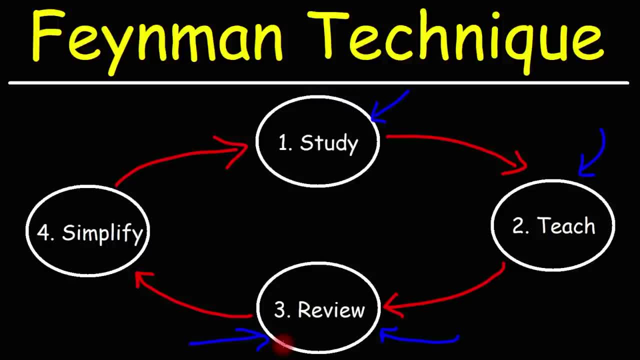 yourself or, even better, to someone else. This will help you to know if you have a good grasp of the topic or if you need to go back and study some more. So that's the basic idea behind Feynman's technique of learning something new, and 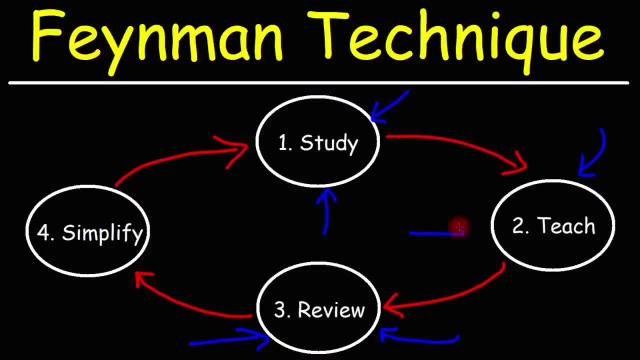 understanding it. Number one: you want to study it. Number two: teach it to others. Number three: once you've identified gaps in your knowledge, go back and review the material. Number four: simplify your explanation. Develop the ability to explain what you learned in such a simple way that. 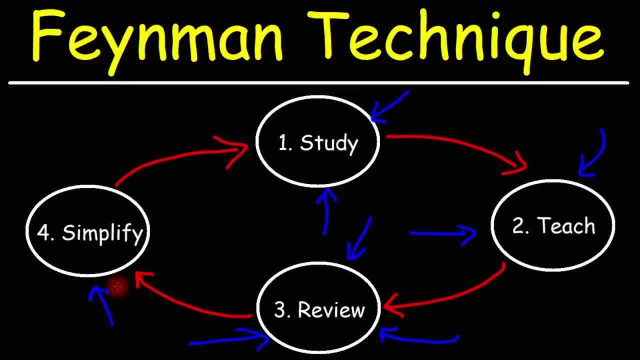 anyone with a limited vocabulary can understand. So that's the basic idea behind Feynman's technique, and hopefully you found this video to be helpful. Now I'm going to take a moment to discuss an ebook that will be very useful for those of